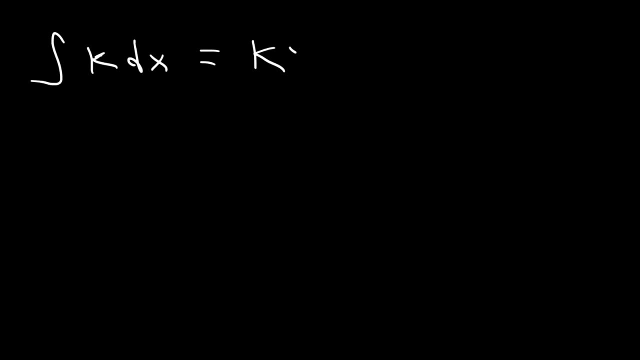 variable of x, this is going to equal kx plus c. So if I want to integrate 5dx, this is going to be 5x plus c. If I wish to integrate, let's say, 12dy, That's going to be 12y plus c, Or 4dt, this is going to be 4t plus c. 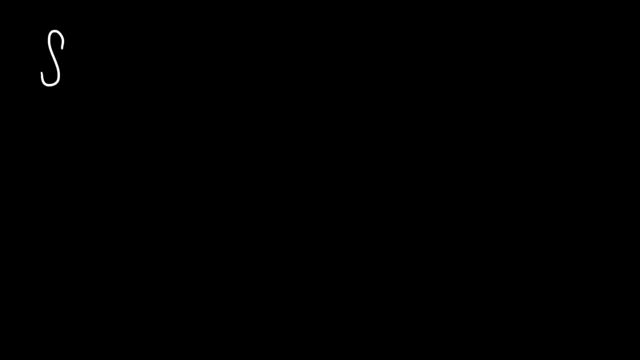 Now another rule that you need to be familiar with is the power rule. The antiderivative of x raised to the n dx is equal to x raised to the n plus 1, divided by n plus 1 plus some constant c. So let me give you some examples of using this power rule. 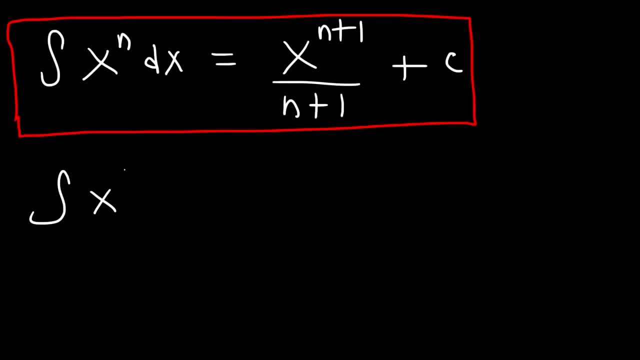 So let's say, if we wish to find the antiderivative of x squared dx, This is going to be x raised to the 2 plus 1 divided by 2 plus 1 plus c. So it's x cubed over 3 plus c, which you could write that as 1. third, x cubed plus c. 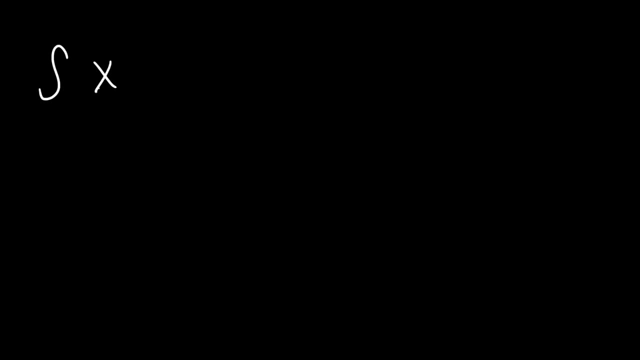 So let's try some more examples using the power rule. Go ahead and find the antiderivative of x cubed, 10x to the 4th. and also, let's say 1 over x squared. Go ahead and try these problems. 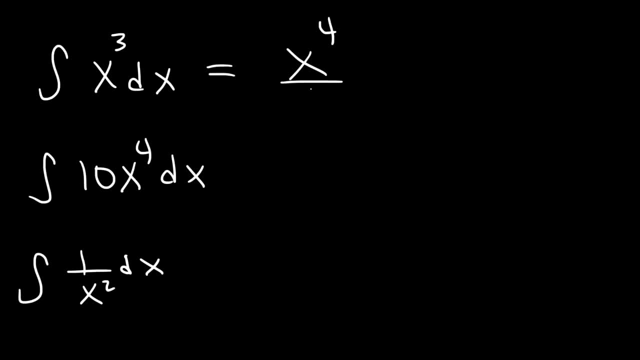 So for this one, 3 plus 1 is 4, so it's going to be x to the 4th over 4 plus c. For the next one, 4 plus 1 is 5, so it's x to the 5th over 5.. 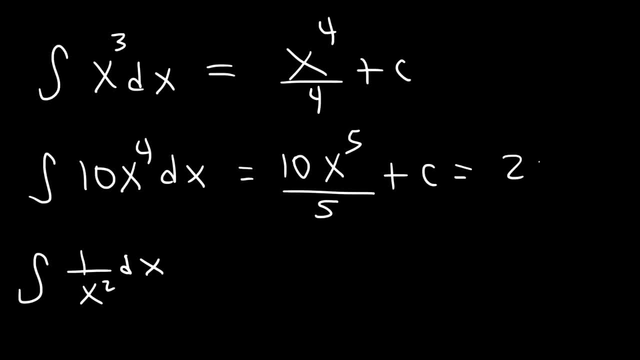 But we could simplify it: 10 divided by 5 is 2.. So it's 2x x to the 5th power plus c. Now what about the last one, 1 over x squared? What can we do for that example? 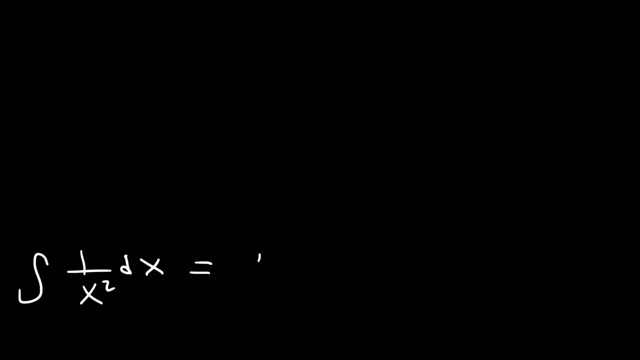 Before you integrate it you need to rewrite it. So we can rewrite it as x raised to the negative 2 dx and then use the power rule. So it's x raised to the negative 2 plus 1 divided by negative 2 plus 1 plus c. 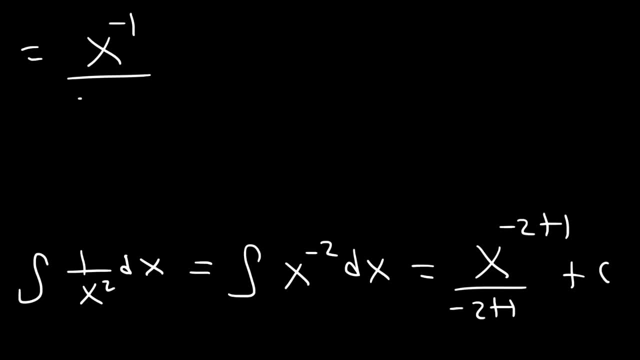 And so negative 2 plus 1 is negative 1.. And then we can rewrite the final answer as negative 1 over x plus c. So anytime you have a rational function like this one, make sure to rewrite it. So let's try another simple example. 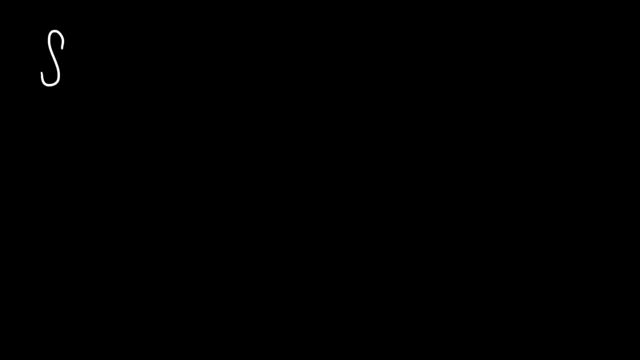 Now another rule that you need to be familiar with is the power rule. The antiderivative of x raised to the n dx is equal to x raised to the n plus 1, divided by n plus 1 plus some constant c. So let me give you some examples of using this power rule. 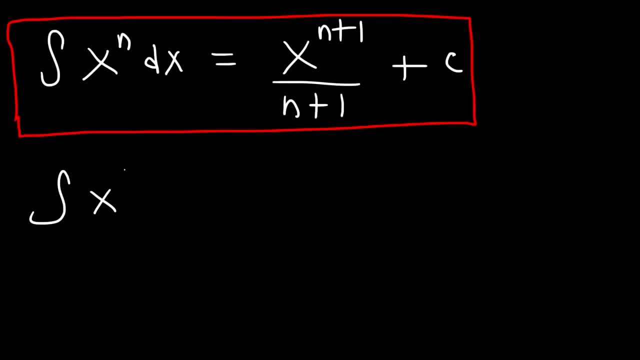 So let's say, if we wish to find the antiderivative of x squared dx, This is going to be x raised to the 2 plus 1 divided by 2 plus 1 plus c. So it's x cubed over 3 plus c, which you could write that as 1. third, x cubed plus c. 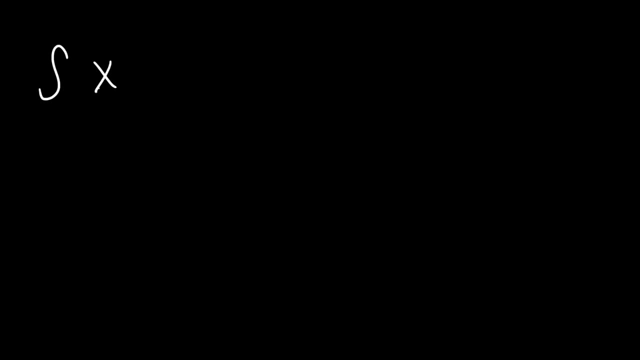 So let's try some more examples using the power rule. Go ahead and find the antiderivative of x cubed, 10x to the 4th. and also, let's say 1 over x squared. Go ahead and try these problems. 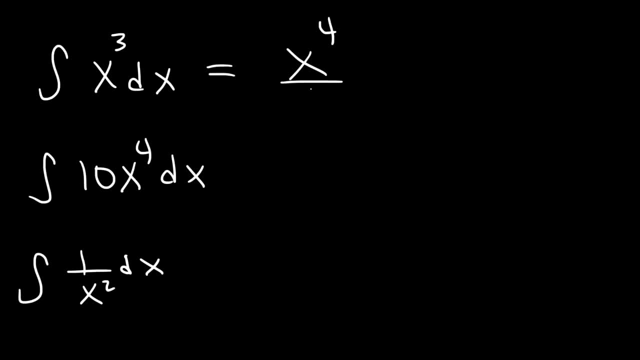 So for this one, 3 plus 1 is 4, so it's going to be x to the 4th over 4 plus c. For the next one, 4 plus 1 is 5, so it's x to the 5th over 5.. 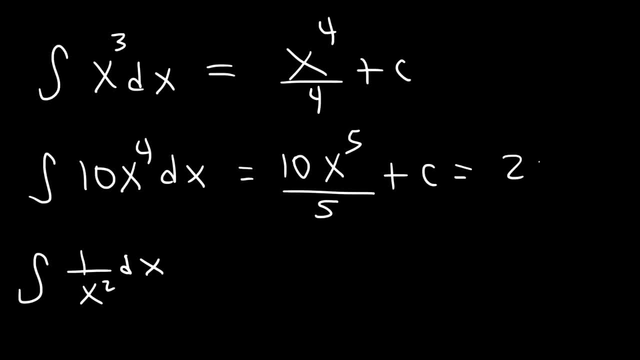 But we could simplify it: 10 divided by 5 is 2.. So it's 2x x to the 5th power plus c. Now what about the last one, 1 over x squared? What can we do for that example? 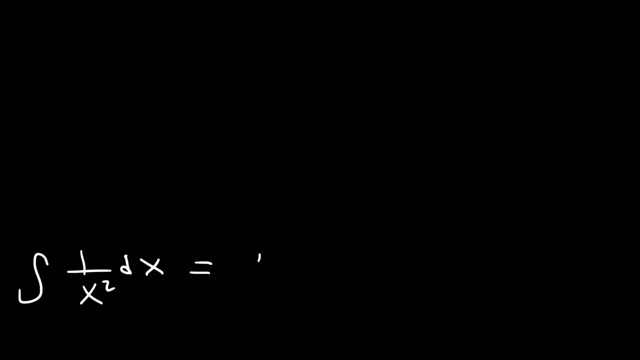 Before you integrate it you need to rewrite it. So we can rewrite it as x raised to the negative 2 dx and then use the power rule. So it's x raised to the negative 2 plus 1 divided by negative 2 plus 1 plus c. 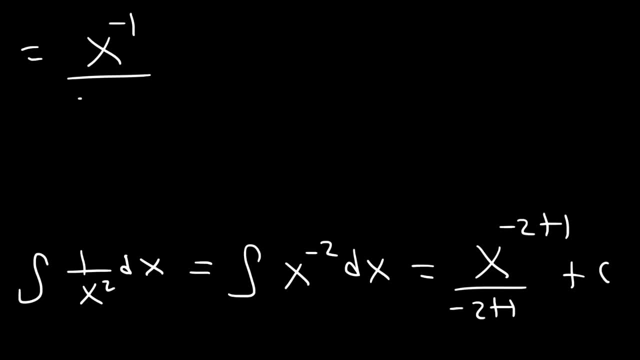 And so negative 2 plus 1 is negative 1.. And then we can rewrite the final answer as negative 1 over x plus c. So anytime you have a rational function like this one, make sure to rewrite it. So let's try another simple example. 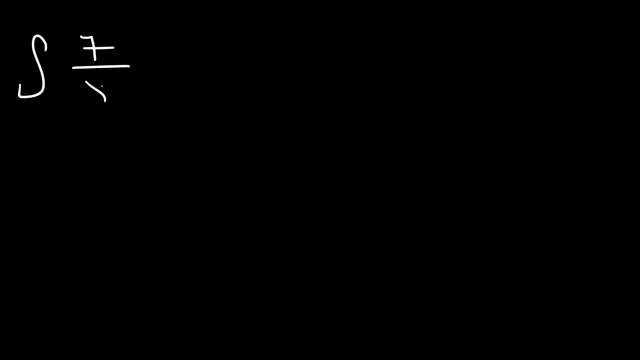 Let's say, if we want to integrate 7 over x to the 4th power, Try that one. So first let's rewrite it as 7x, x raised to the negative 4.. And then let's use the power rule. 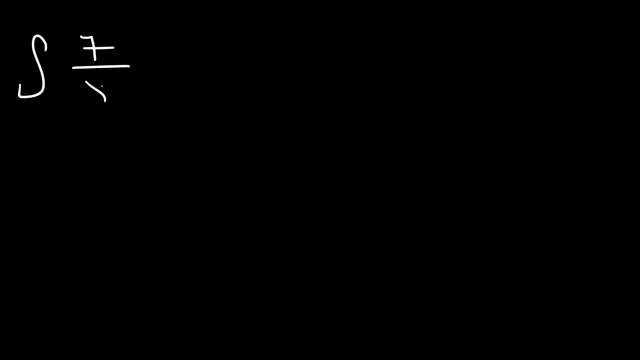 Let's say, if we want to integrate 7 over x to the 4th power, Try that one. So first let's rewrite it as 7x, x raised to the negative 4.. And then let's use the power rule. 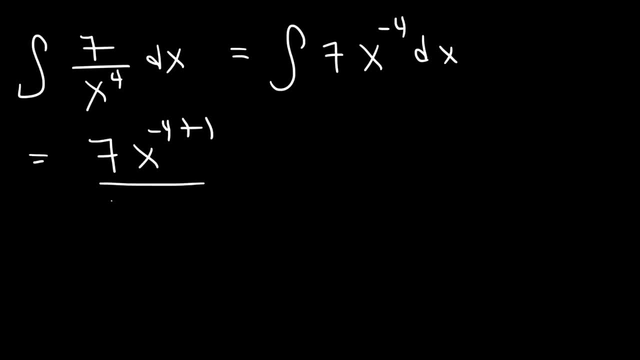 So it's going to be negative 4 plus 1 divided by negative 4 plus 1 plus c, And negative 4 plus 1 is negative 3.. So then this is equal to negative 7 divided by 3x, to the 3rd power plus c. 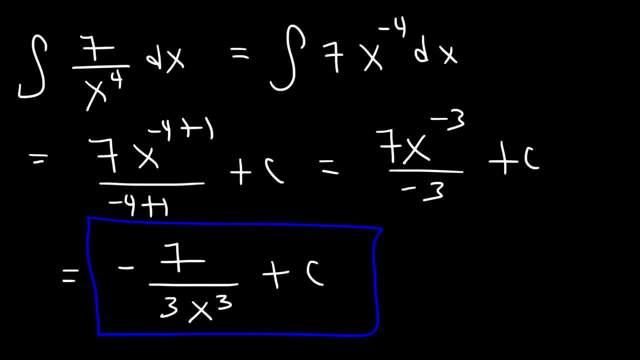 And that's the final answer. Now you can also use the power rule when integrating radical functions. Let's say, if we want to find the antiderivative of the cube root of x, So first you need to rewrite it. This is x to the 1- 3rd. 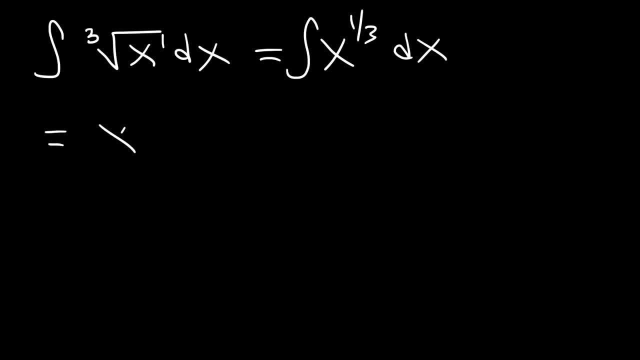 And then use the power rule. So this is going to be x raised to the 1, 3rd plus 1, divided by 1, 3rd plus 1 plus c, So 1, 3rd plus 1.. We need to get common denominators. 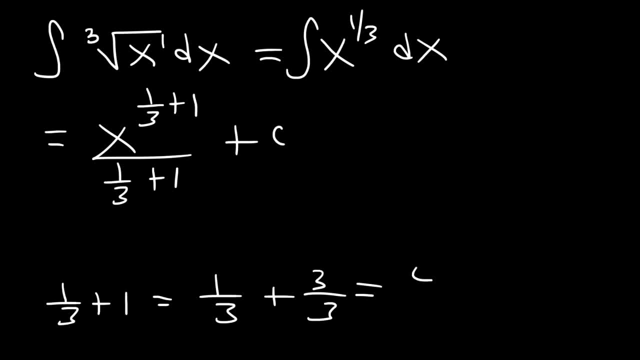 And 1 is the same as 3. And 1 plus 3 is 4.. So we can rewrite this as: x raised to the 4 3rds, divided by 4 over 3 plus c. Now we can multiply the top and the bottom by the reciprocal of 4 over 3.. 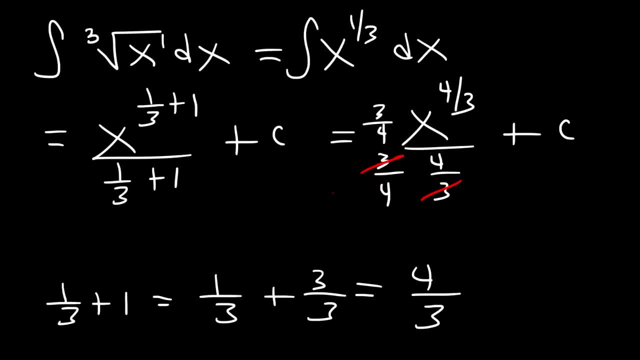 And that is 3 4ths. So on the bottom the 3s will cancel and the 4s will cancel. So we can rewrite the final answer as 3 4ths x raised to the 4 over 3 plus c. 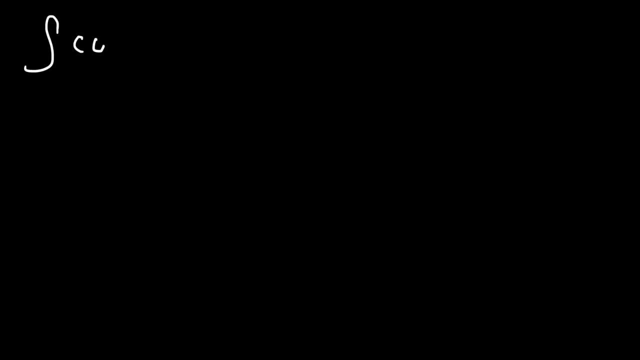 Now let's go over the antiderivatives of six trigonometric functions. The antiderivative of cosine x is sine x. You should write these down and commit them to memory. The antiderivative of sine x is negative cosine x. 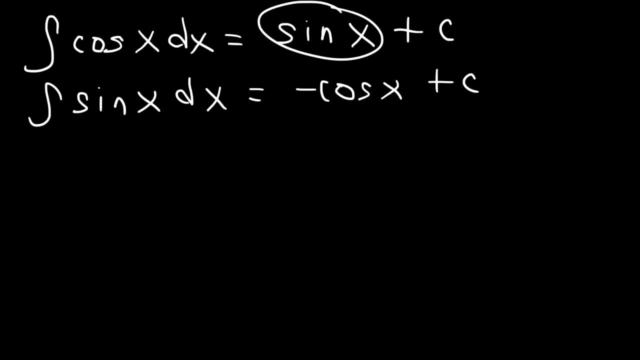 Now keep in mind: if you know the derivative, then you can know the derivative, You can know the antiderivative. The derivative of sine is cosine. The derivative of cosine is negative sine. So the derivative of negative cosine is positive sine. 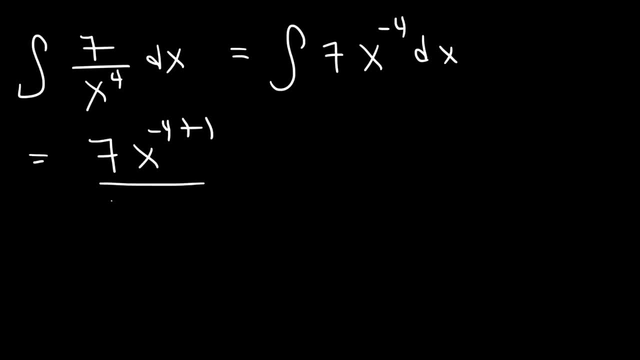 So it's going to be negative 4 plus 1 divided by negative 4 plus 1 plus c, And negative 4 plus 1 is negative 3.. So then this is equal to negative 7 divided by 3x, to the 3rd power plus c. 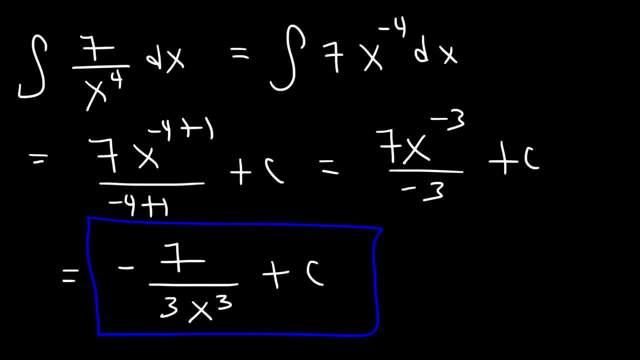 And that's the final answer. Now you can also use the power rule when integrating radical functions. Let's say, if we want to find the antiderivative of the cube root of x, So first you need to rewrite it. This is x to the 1- 3rd. 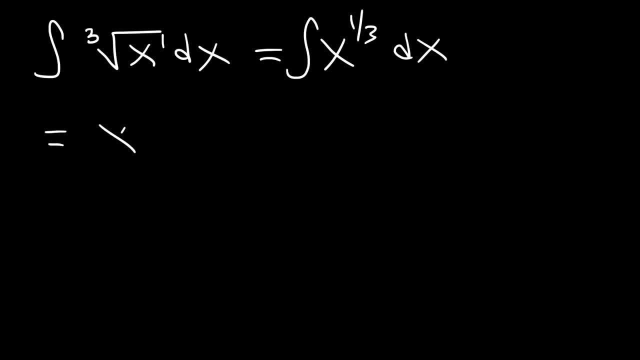 And then use the power rule. So this is going to be x raised to the 1, 3rd plus 1, divided by 1, 3rd plus 1 plus c, So 1, 3rd plus 1.. We need to get common denominators. 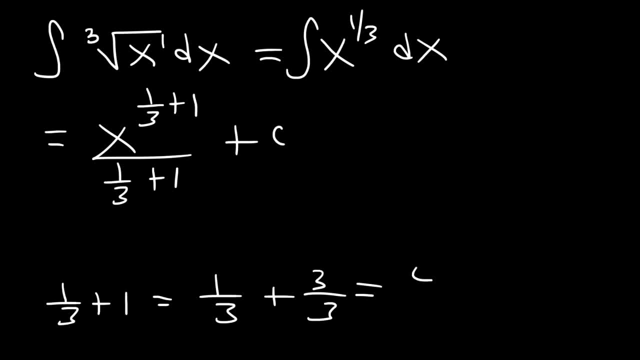 And 1 is the same as 3. And 1 plus 3 is 4.. So we can rewrite this as: x raised to the 4 3rds, divided by 4 over 3 plus c. Now we can multiply the top and the bottom by the reciprocal of 4 over 3.. 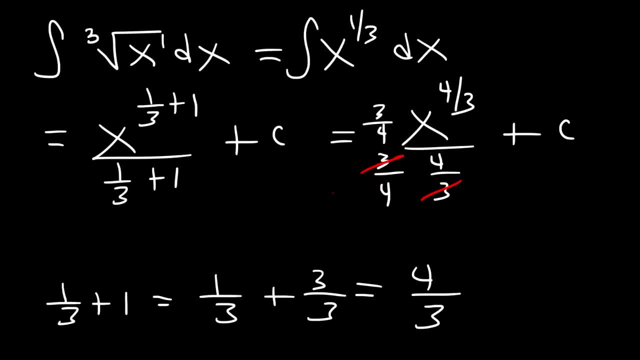 And that is 3 4ths. So on the bottom the 3s will cancel and the 4s will cancel. So we can rewrite the final answer as 3 4ths x raised to the 4 over 3 plus c. 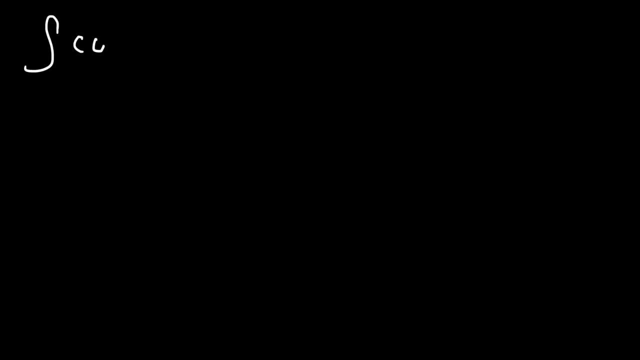 Now let's go over the antiderivatives of six trigonometric functions. The antiderivative of cosine x is sine x. You should write these down and commit them to memory. The antiderivative of sine x is negative cosine x. 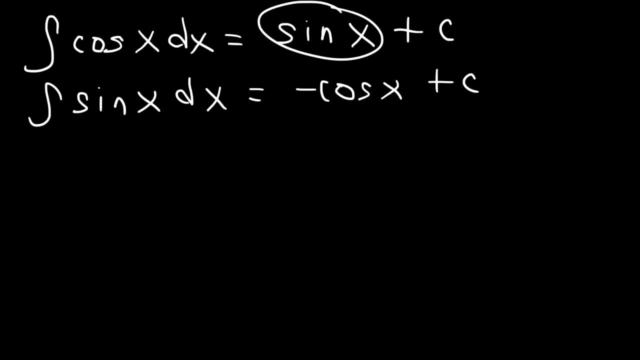 Now keep in mind: if you know the derivative, then you can know the derivative, You can know the antiderivative. The derivative of sine is cosine. The derivative of cosine is negative sine. So the derivative of negative cosine is positive sine. 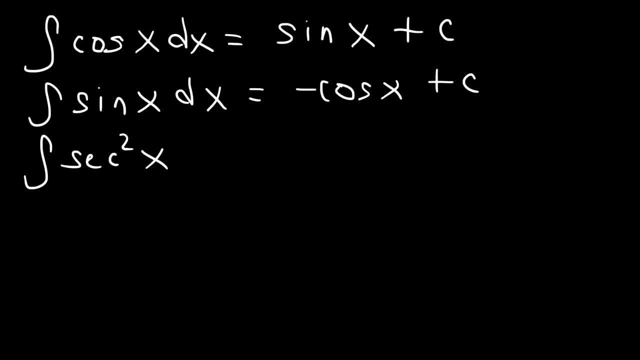 Now the antiderivative of secant squared, that's equal to tangent x, And the antiderivative of secant x, tangent x, dx, that's going to be secant x plus c, And the antiderivative of cosecant squared. 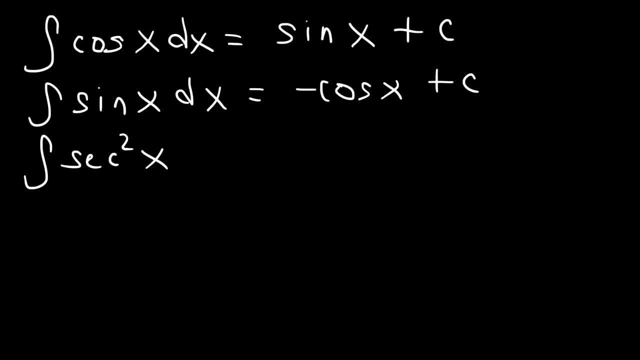 Now the antiderivative of secant squared, that's equal to tangent x, And the antiderivative of secant x, tangent x, dx, that's going to be secant x plus c, And the antiderivative of cosecant squared. 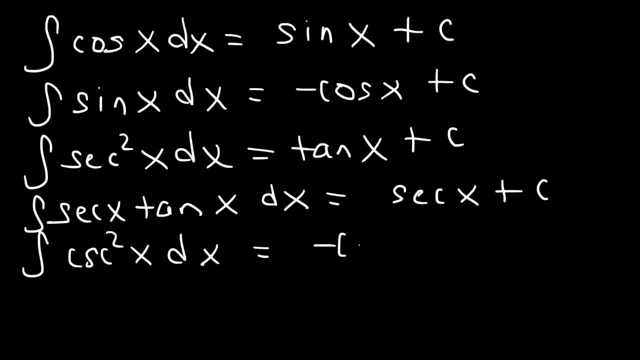 is going to be negative cotangent x plus c And the antiderivative of cosecant x, cotangent x. that's negative cosecant x plus c. So hopefully you had a chance to write that down. Now let's work on some example problems. 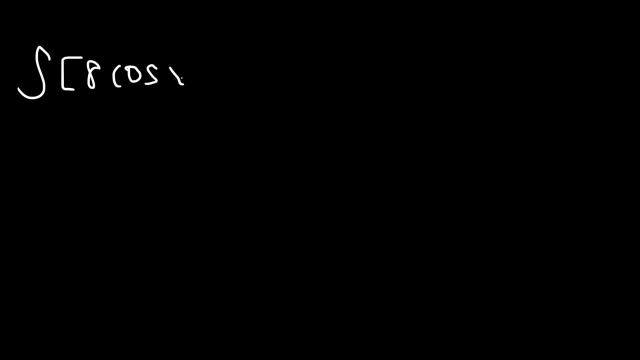 Go ahead and integrate this function: 8 cosecant x, 8 cosecant x plus 3 cosecant x dx. So the antiderivative of cosine we said is sine. So this is going to be 8 times sine. 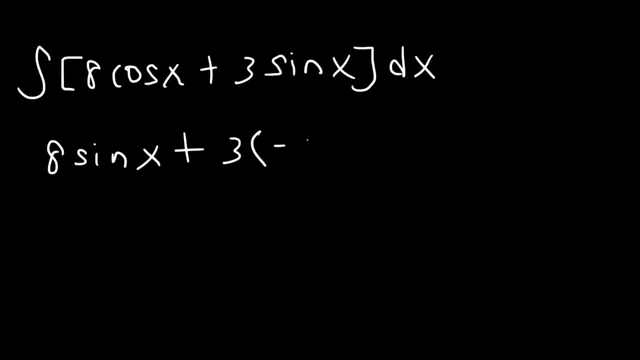 And the antiderivative of sine is negative cosine, And let's not forget to add plus c. So the final answer is 8 cosecant x minus 3 cosecant x plus c, And so if you know the derivative, it's very easy to integrate trigonometric functions. 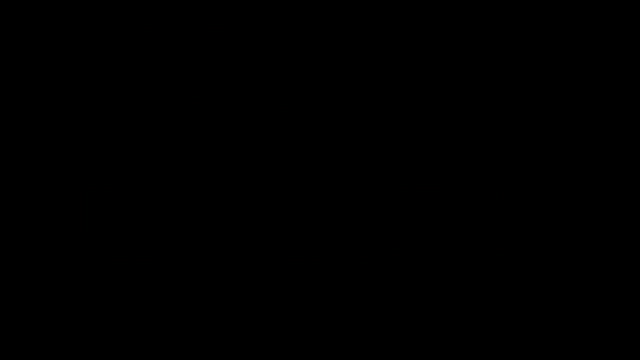 that look like this. Here's another one that you could try. Find the antiderivative of 4: secant squared x minus secant x, tangent x. So the antiderivative of secant squared- we know it's tangent x- And the antiderivative of secant tan. 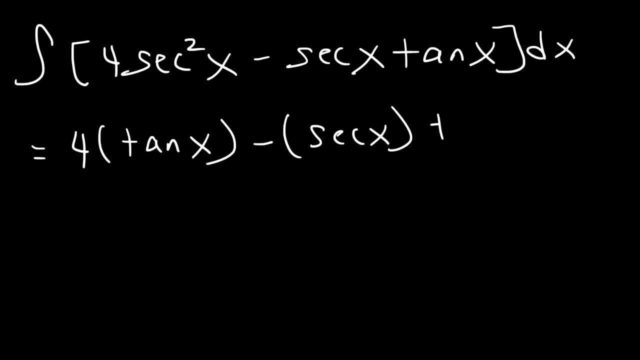 is secant x. So this is the answer: It's 4 tangent x minus secant x, plus the constant of integration c. Let's work on one more example with regards to trig functions. Let's integrate cosecant x times cotangent x minus cosecant x. 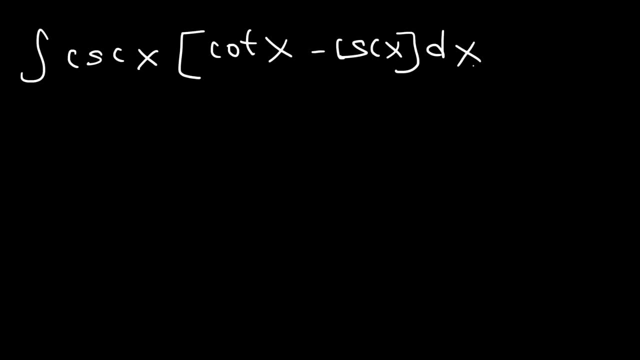 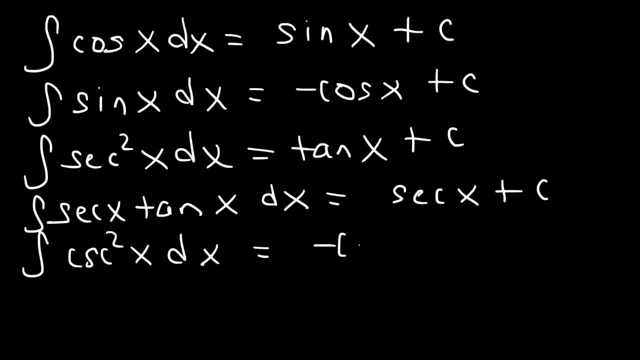 is going to be negative cotangent x plus c And the antiderivative of cosecant x, cotangent x. that's negative cosecant x plus c. So hopefully you had a chance to write that down. Now let's work on some example problems. 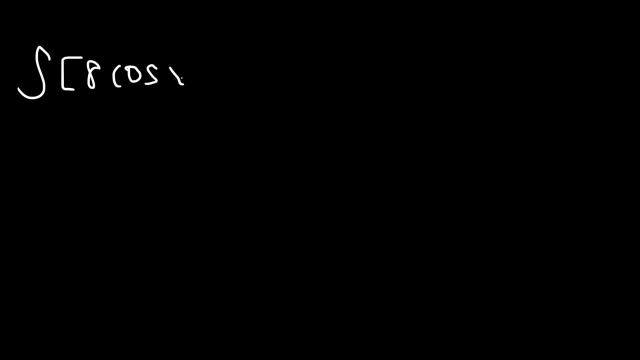 Go ahead and integrate this function: 8 cosecant x, 8 cosecant x plus 3 cosecant x dx. So the antiderivative of cosine we said is sine. So this is going to be 8 times sine. 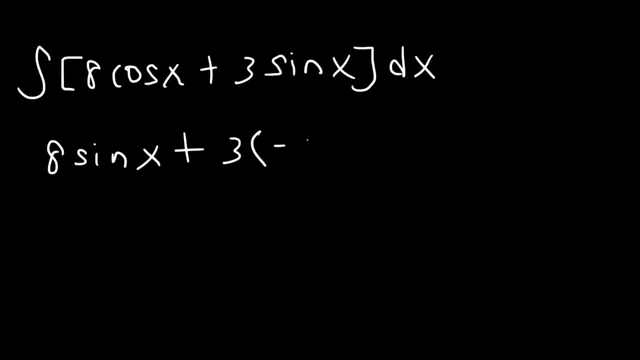 And the antiderivative of sine is negative cosine, And let's not forget to add plus c. So the final answer is 8 cosecant x minus 3 cosecant x plus c, And so if you know the derivative, it's very easy to integrate trigonometric functions. 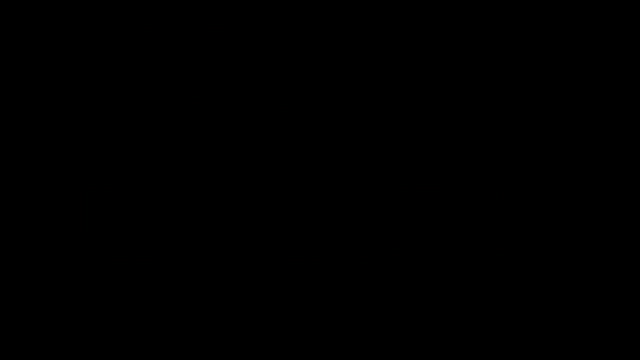 that look like this. Here's another one that you could try. Find the antiderivative of 4: secant squared x minus secant x, tangent x. So the antiderivative of secant squared- we know it's tangent x- And the antiderivative of secant tan. 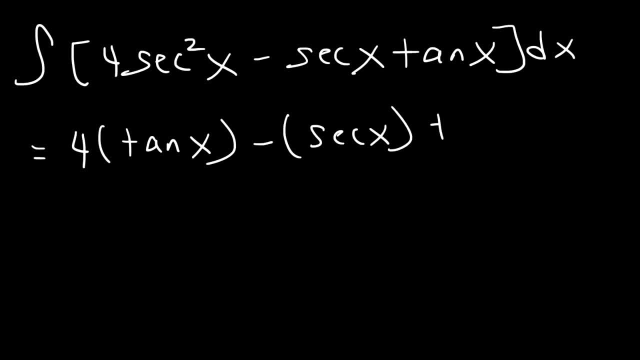 is secant x. So this is the answer: It's 4 tangent x minus secant x, plus the constant of integration c. Let's work on one more example with regard to trig functions. Let's integrate cosecant x times cotangent x. 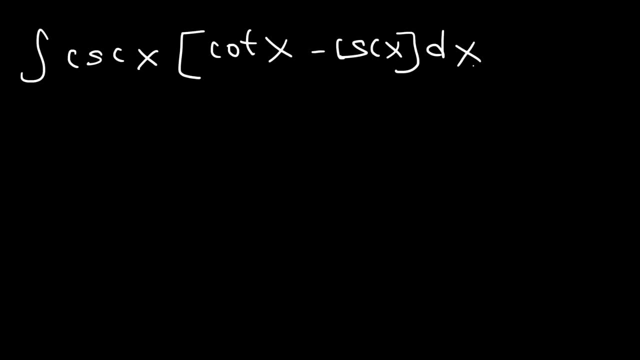 minus cosecant x. Now for this particular example, we need to rewrite it before we integrate it. Let's distribute cosecant to cotangent minus cosecant, So cosecant times cotangent, that's just cosecant cotangent. We still have the integration symbol. 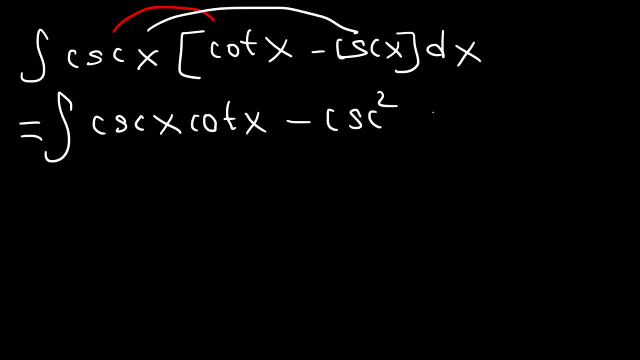 And then cosecant times cosecant is cosecant squared. Now the antiderivative of cosecant cotangent is negative cosecant x, And the antiderivative of cosecant squared is negative cotangent x. So the final answer is gonna be: Let's distribute cosecant to cotangent minus cosecant. Let's distribute cosecant to cotangent minus cosecant. Let's distribute cosecant to cotangent minus cosecant. So cosecant times cotangent, that's just cosecant cotangent. 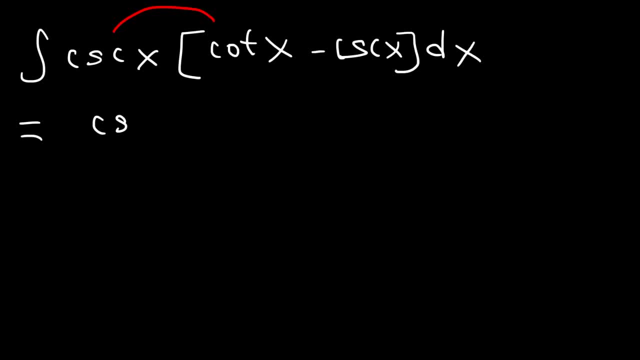 So cosecant times cotangent, that's just cosecant cotangent. So cosecant times cotangent, that's just cosecant cotangent cotangent, that's just cosecant cotangent. we still have the integration symbol. and then cosecant times cosecant is cosecant squared. now the antiderivative of: 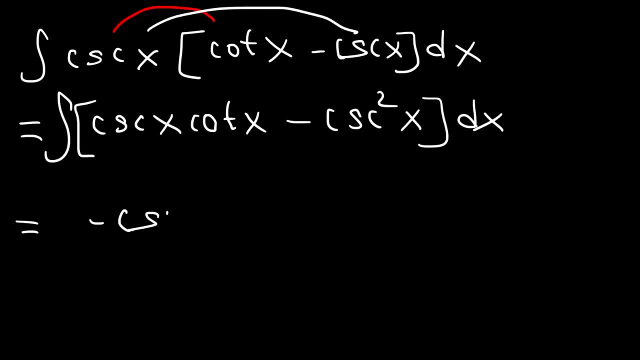 cosecant cotangent is negative cosecant X and the antiderivative of cosecant squared is negative cotangent X. so the final answer is going to be: I'm going to reverse these two, so I have positive cotangent x and negative cosecant X. this part is positive because we have two negative sides. 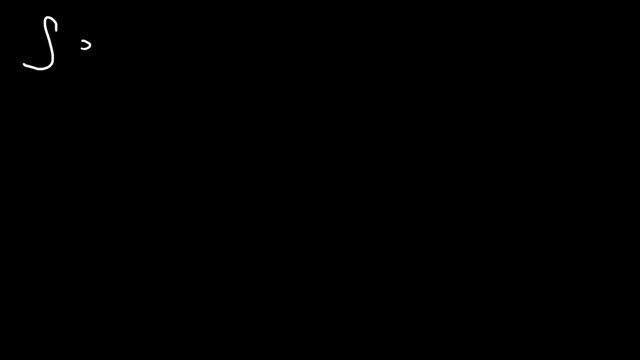 now let's talk about integrating exponential functions. like each of you, it's going to be E to the U divided by u prime plus C. if U is a little under hell, linear function, or if u prime is a constant. If u prime is not a constant, this will not work. 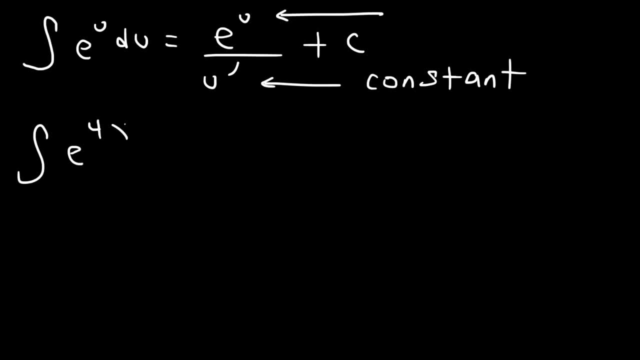 So let's work on some examples. Let's say, if we want to integrate e to the 4x, It's going to be the same thing: e to the 4x divided by the derivative of 4x, which is 4.. 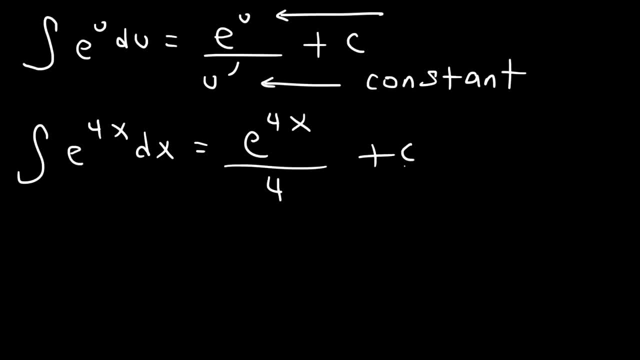 Because this is a constant, this will be the right answer. Now, let's say, if we want to integrate e to the 7x minus 3.. Let's not forget dx. So it's going to be the same thing: e to the 7x minus 3,. 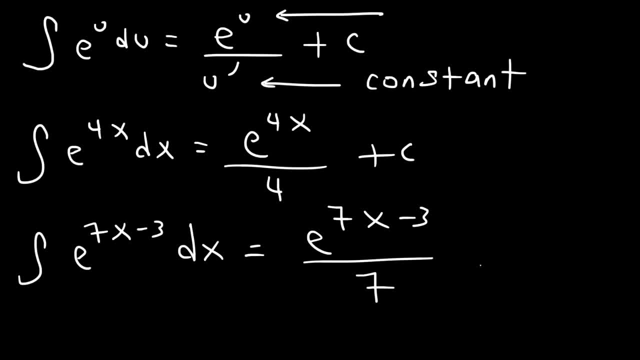 and the derivative of 7x minus 3 is a constant like 7,, and so that's going to be the answer. Now let's say if we want to integrate e to the x, It's going to be the same thing. 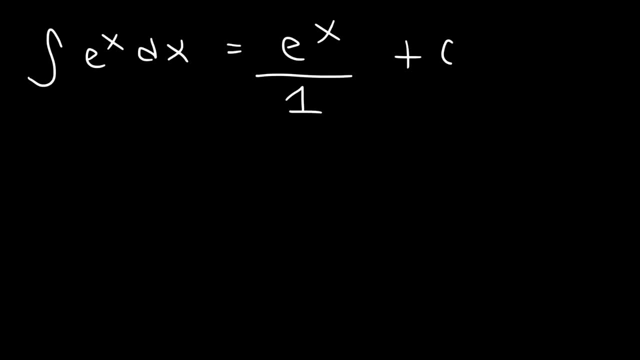 divided by the derivative of x, which is 1.. So it's simply e to the x plus some constant c. Now, this one, This one won't work. We can't say it's e to the x squared divided by 2x. This is not a constant. 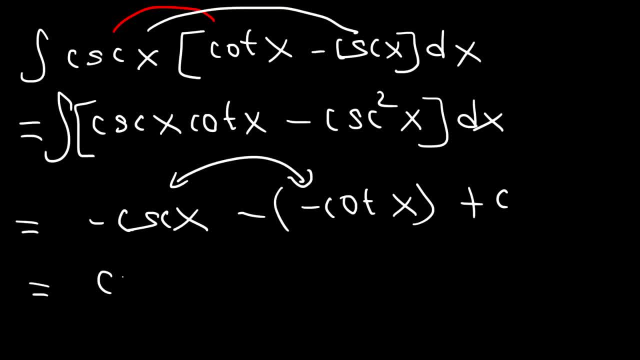 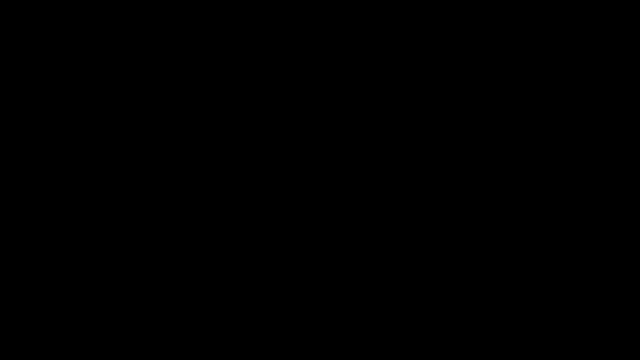 I'm gonna reverse these two, So I have positive cotangent x and negative cosecant x. This part is positive because we have two negative signs. Now let's talk about integrating exponential functions like e to the? u. It's gonna be e to the? u divided by u prime plus c. 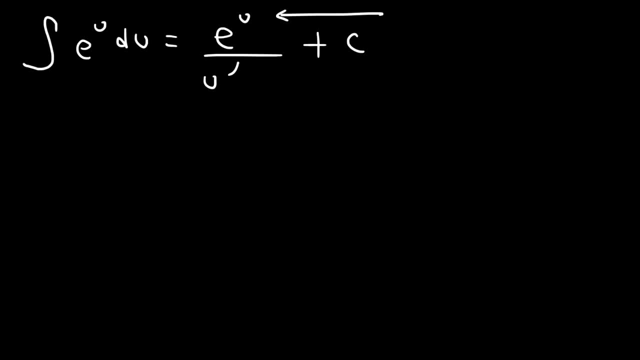 if u is a linear function or if u prime is a constant. If u prime is not a constant, this will not work. So let's work on some examples. Let's say, if we want to integrate e to the four x, It's gonna be the same thing e to the four x. 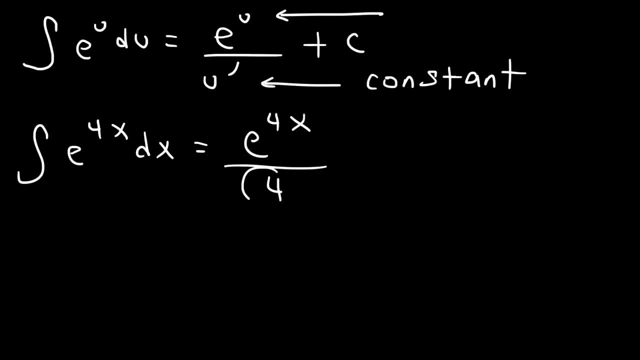 divided by the derivative of four, x, which is four, Because this is a constant, this will be the right answer. Now let's say, if we want to integrate e to the seven x minus three, Let's not forget dx, So it's gonna be the same thing: e to the seven x minus three. 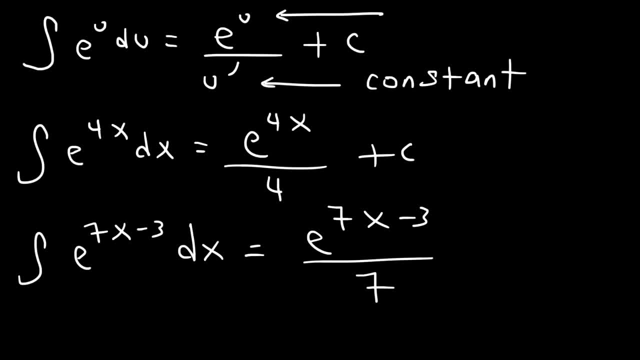 And the derivative of seven x minus three is a constant like seven, And so that's gonna be the answer. Now let's say, if we want to integrate e to the x, It's gonna be the same thing divided by the derivative of x, which is one. 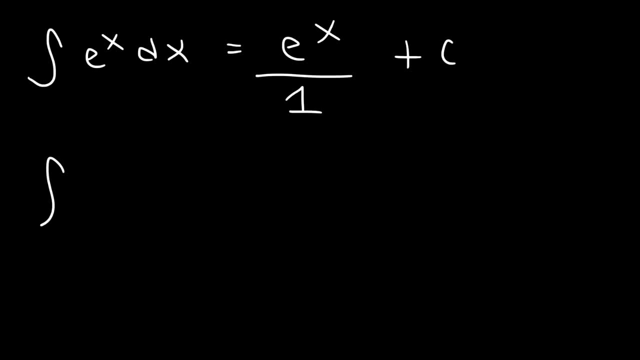 So it's simply e to the x plus some constant c. Now this one won't work. We can't say it's e to the x squared divided by two x. This is not a constant. So in this situation this will not be the answer. 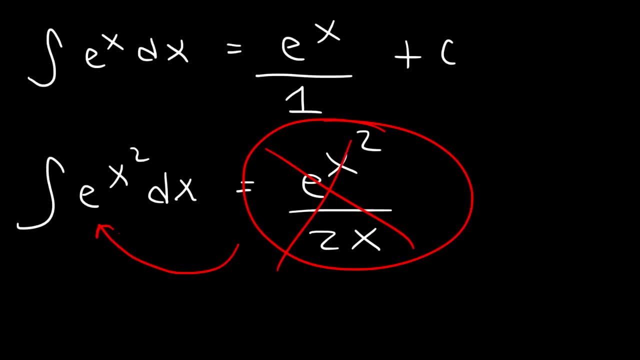 If you try to find the derivative of this expression, it will not give you e to the x squared. Now let's move on to logarithmic functions. The antiderivative of one over u du is going to be the natural log of u divided by u prime. 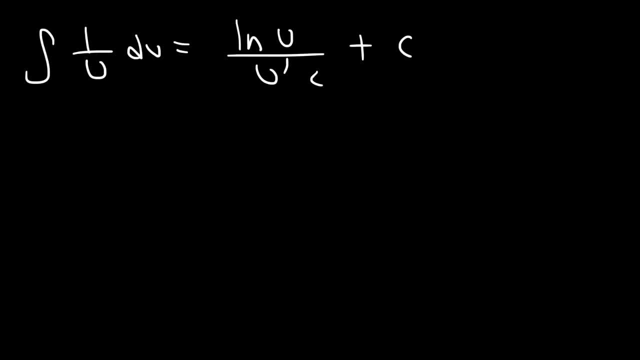 And the same is true. U has to be a linear function and u prime must be a constant. If it's a variable, it won't work. So let's say, if we want to find the antiderivative of one over x. 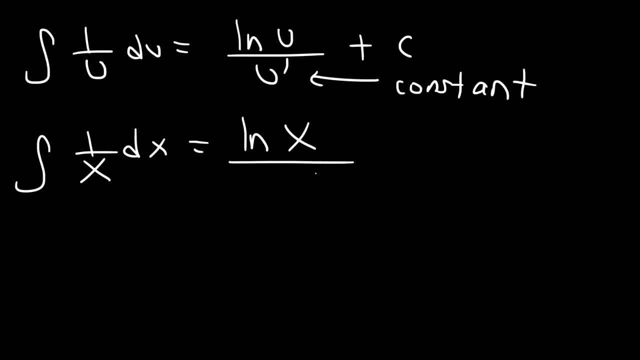 It's gonna be ln x divided by the derivative of x, which is one plus c. So let's say, if we want to integrate one over x plus five, It's going to be the natural log of x plus five and the derivative of x plus five is one. 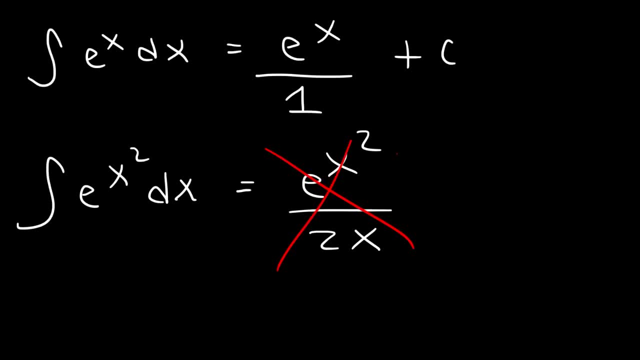 So in this situation, this will not be the answer. If you try to find the derivative of this expression, it will not give you e to the x squared. Now let's move on to logarithmic functions. The antiderivative of 1 over u du is going to be the natural log of u divided by u prime. 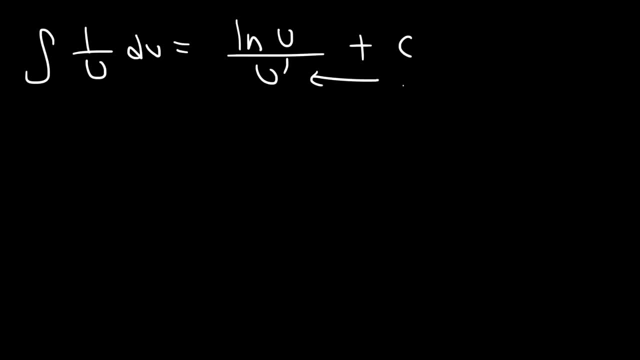 And the same is true. u has to be a linear function and u prime must be a constant. If it's a variable, it won't work. So let's say, if we want to find the antiderivative of 1 over x, 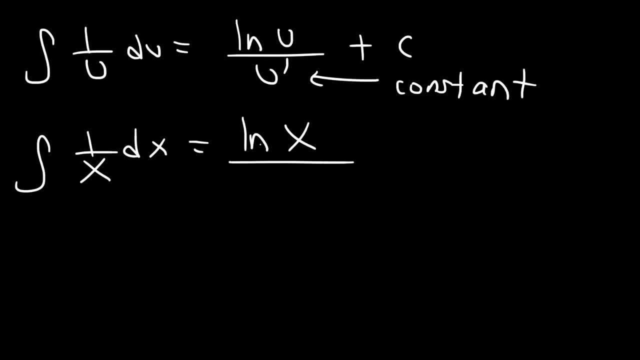 It's going to be ln, x divided by the derivative of x, which is 1, plus c. So let's say, if we want to integrate 1 over x plus 5. It's going to be the natural log of x plus 5, and the derivative of x plus 5 is 1.. 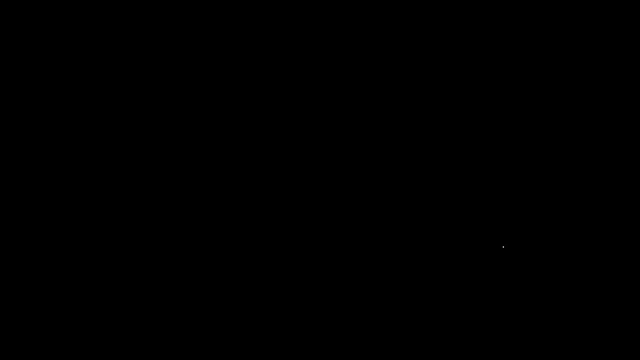 And so it's just. It's ln, x plus 5, plus c. Now try this one: What's the antiderivative of 1 over 4x minus 3?? So it's going to be the natural log of 4x minus 3, and the derivative of 4x minus 3 is 4.. 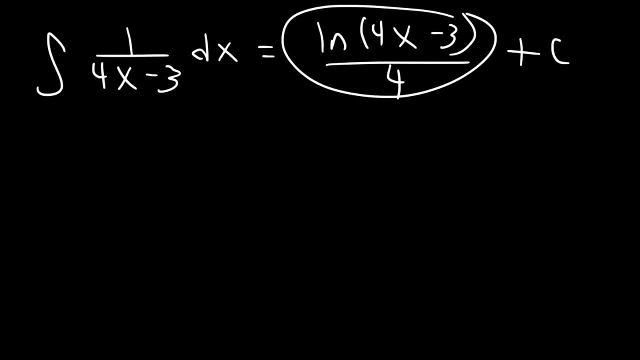 Now let's confirm the answer, Let's find the derivative of this expression. So if we were to differentiate 1, fourth natural log, 4x minus 3, well, we get the original answer, The original problem. I mean To differentiate the natural log of u. it's equal to u prime over u. 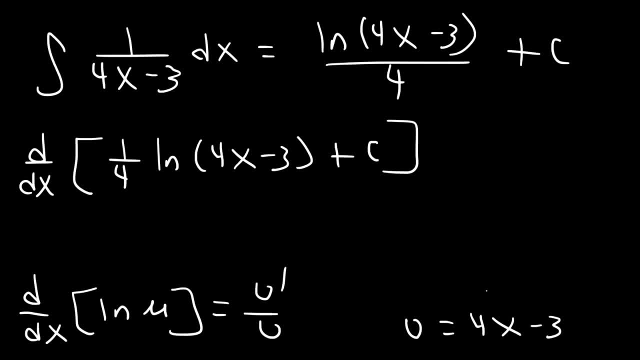 So in this case u is 4x minus 3, and u prime is 4.. So this is going to be 1 fourth, and then u prime over u, so 4 over 4x minus 3.. And the derivative of 4x minus 3 is 4.. 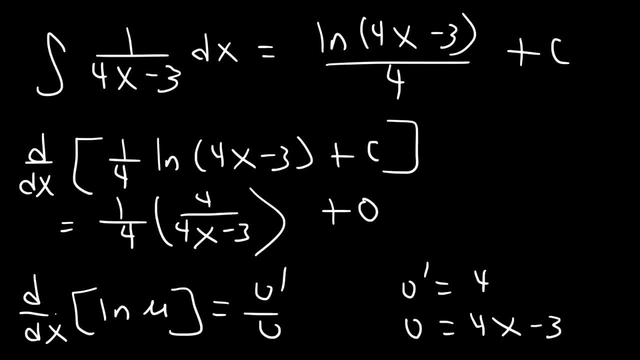 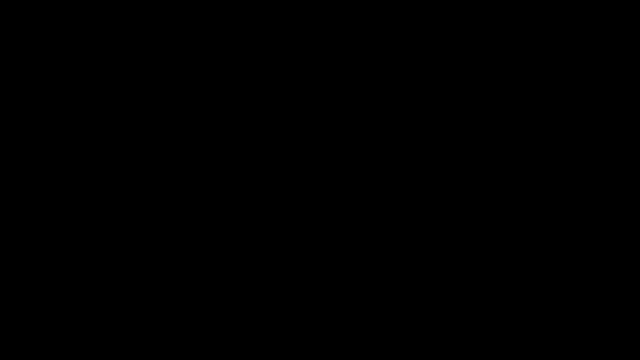 And the derivative of a constant is going to be 0. So in this case the 4s will cancel, and so this will give us the original problem: 1 over 4x minus 3.. And so it works. Let's try one more example. 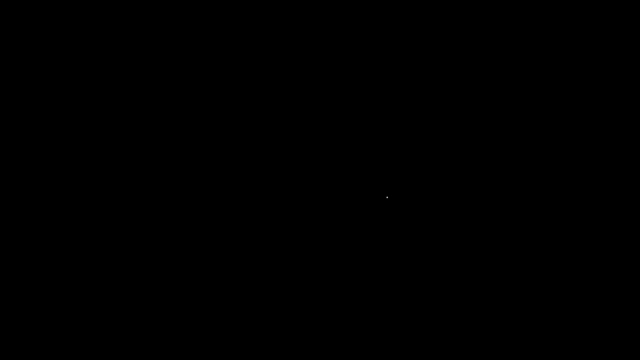 And so it's just ln x plus five plus c. Now try this one: What's the antiderivative of one over four x minus three? So it's going to be the natural log of four x minus three, and the derivative of four x minus three is four. 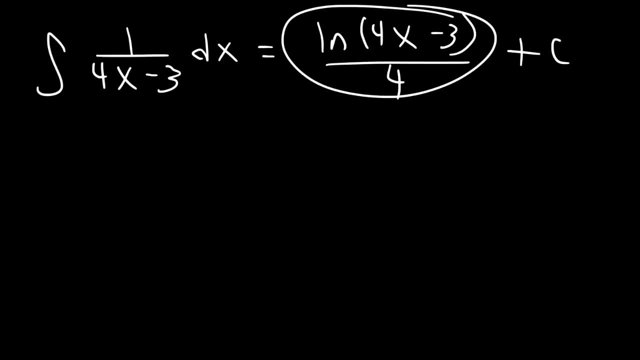 Now let's confirm the answer, Let's find the derivative of this expression. So if we were to differentiate one fourth natural log, four x minus three, well, we get the original answer, The original problem. I mean To differentiate the natural log of u. 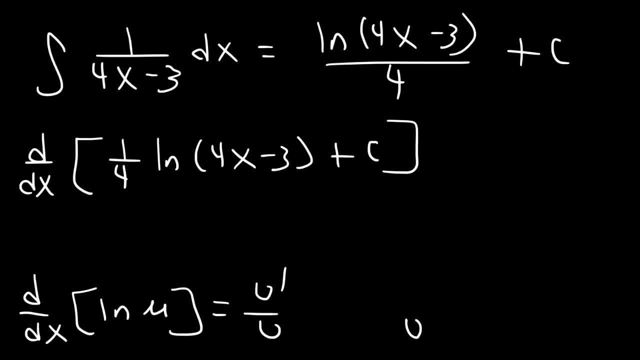 it's equal to u prime over u. So in this case u is four x minus three and u prime is four. So this is gonna be one fourth and then u prime over u, so four over four x minus three, and the derivative of a constant is gonna be zero. 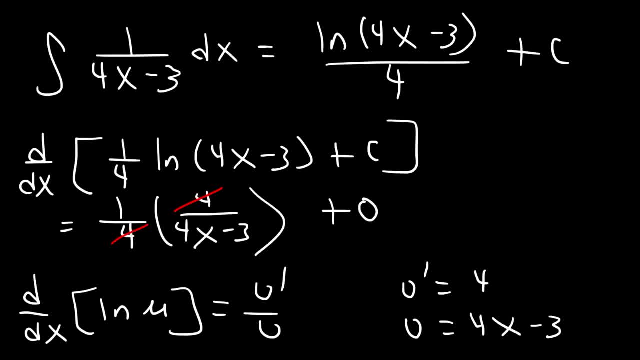 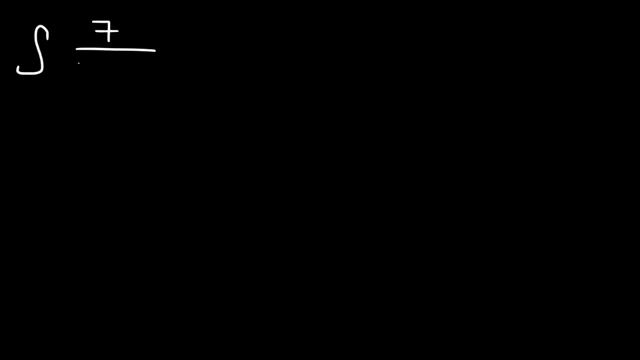 So in this case the fours will cancel, and so this will give us the original problem: one over four x minus three, And so it works. Let's try one more example. What is the antiderivative of seven over three x minus eight times dx? 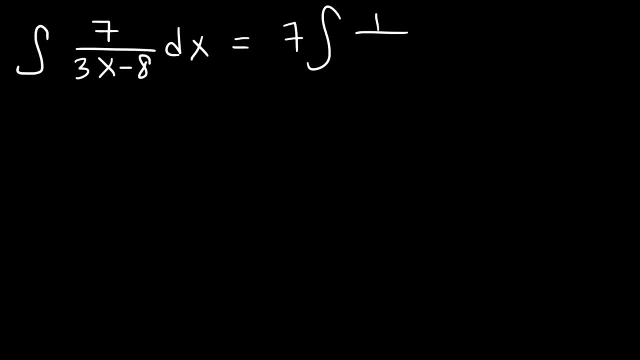 So what I'm gonna do is move the constant seven To the front and then apply the same process in the last problem. So u is going to be 3x minus 8. So then this is going to be 7 times ln of u, or ln of 3x minus 8. 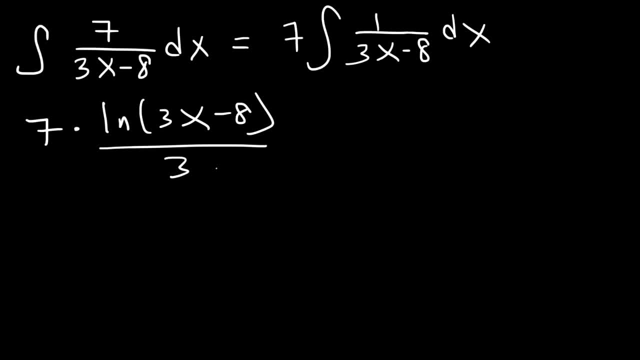 Divided by the derivative of 3x minus 8, which is 3 plus C. So the final answer is going to be 7 over 3 natural log 3x minus 8 plus C. So that's it, and let's confirm it with differentiation. 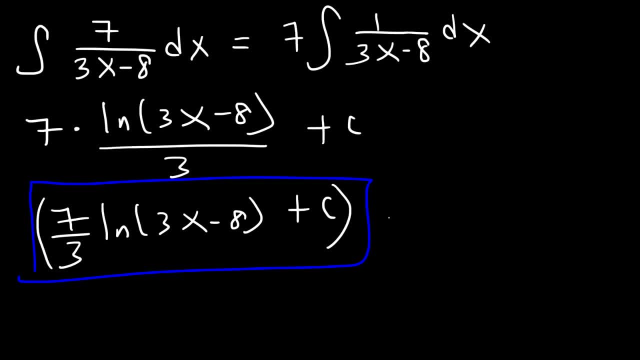 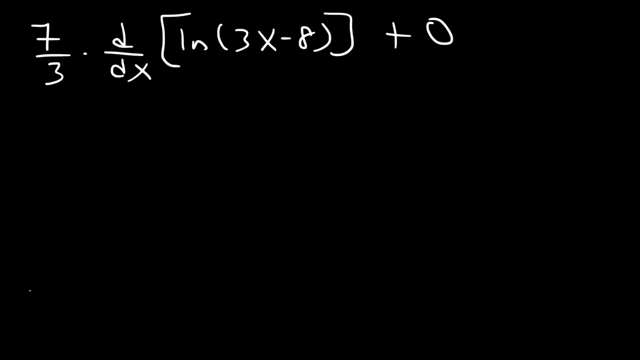 So let's find the derivative of this expression. So it's going to be 7 thirds times the derivative of ln 3x minus 8 and the derivative of C is 0. So in this case, once again, we need to apply This formula. the derivative of ln u is